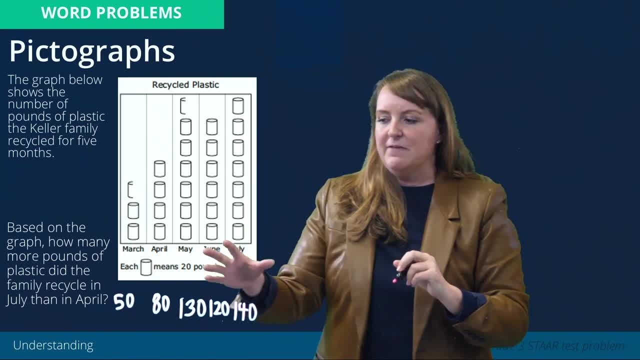 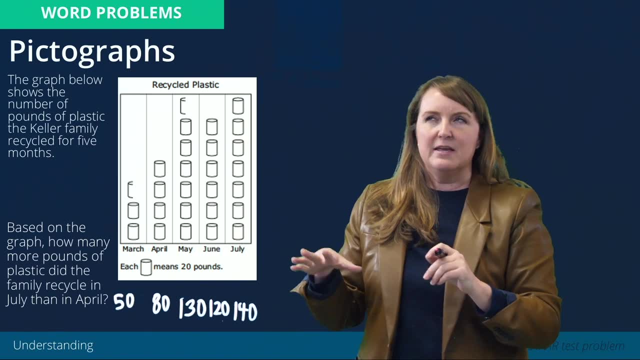 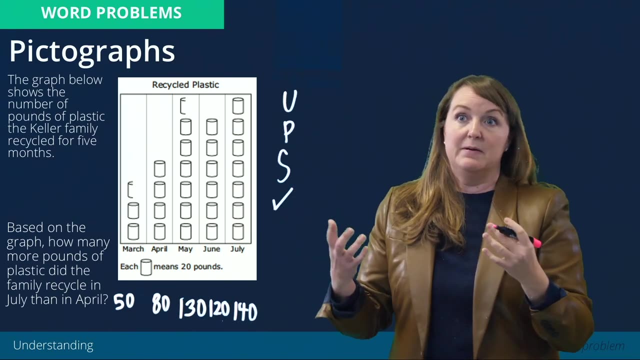 the other months. So now that I have those labeled, if I need that information by month, it's just very easily accessible. So now I've got a word problem and I think, well, whenever I see a word problem, I'm going to U-P-S check that problem. Let's understand this problem by reading. 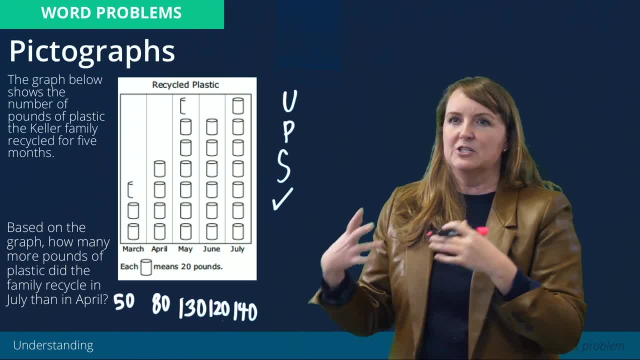 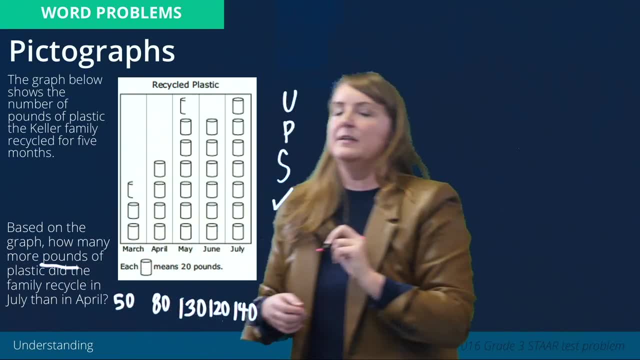 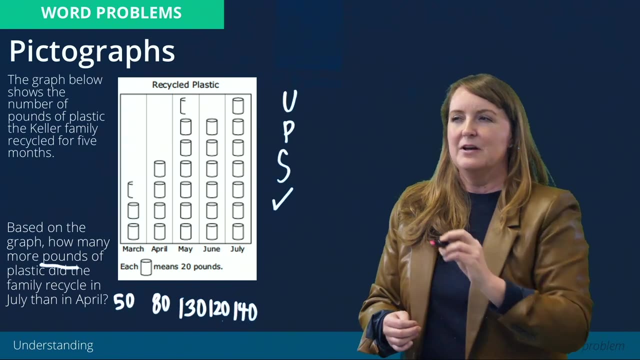 it. How many more pounds of plastic did the family recycle in July than April? So in this problem I have to focus on the number of pounds that that family recycled. I'll go ahead and underline that right there And here are some of the data related to pounds that were recycled. So I 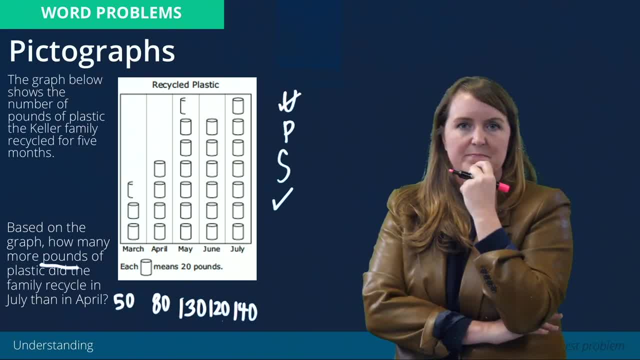 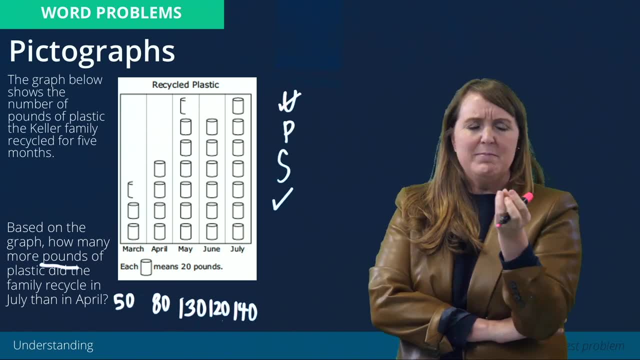 have a pretty good understanding of this problem. Now it's time to make my plan. Is this a total problem, where parts are put together for a total? No, I'm not combining July and April. So then I ask my question: Is this a difference problem? 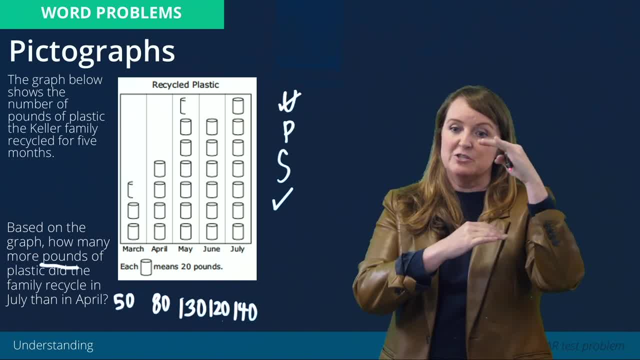 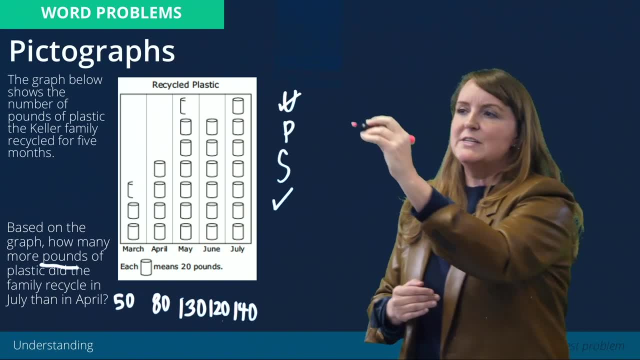 Are amounts compared for a difference, And maybe I use that gesture to sew a greater amount, a lesser amount and a difference And I say, yeah, I'm comparing those two amounts. Once I decide that that I'm going to solve this as a difference problem, I'll go ahead and write. 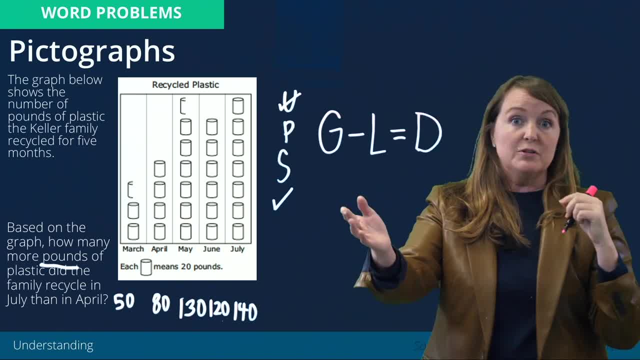 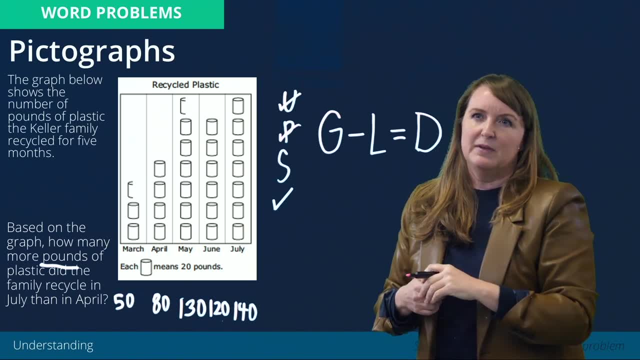 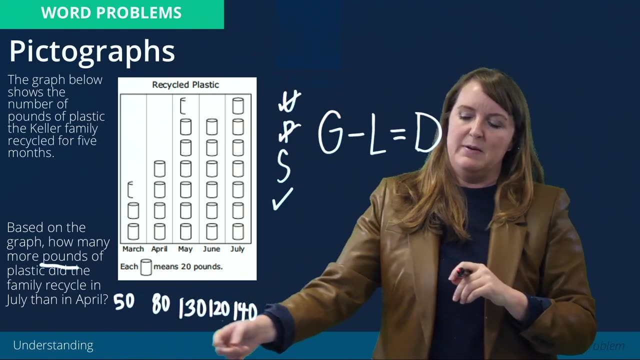 in my difference equation, just like you see here. I could also draw the difference graphic organizer. That would work well as well. But now I've got my plan. Let's solve this as a difference problem. So in, let's see in, July than April. So July had 140 pounds, April had 80 pounds. Let's see July. 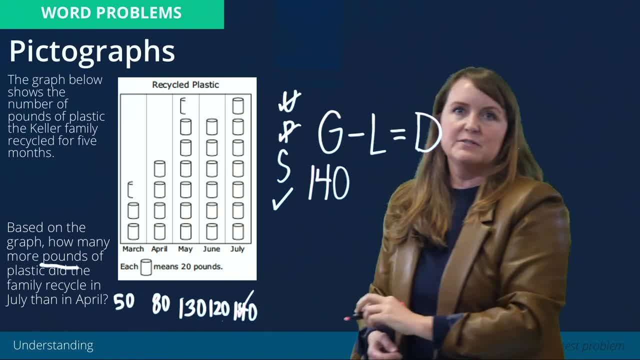 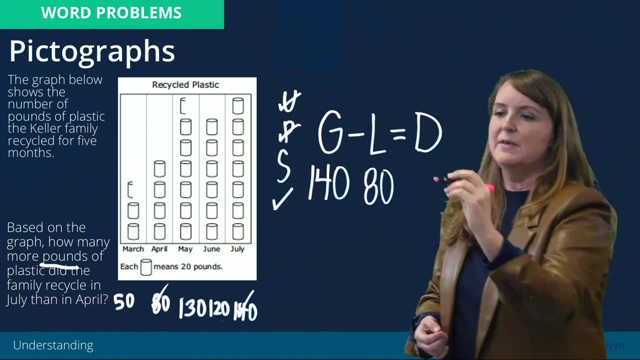 is a greater amount, I'll go ahead and write it right here. I'm going to check that off, so I don't use that again. And 80 is the lesser amount, So I'll go ahead and write that right there And checked it off, so I don't use it again. And we have to figure out the difference. 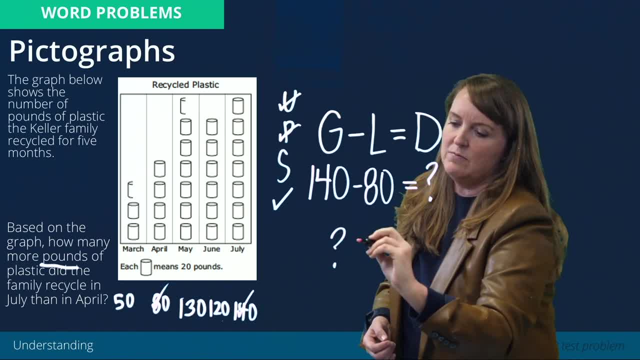 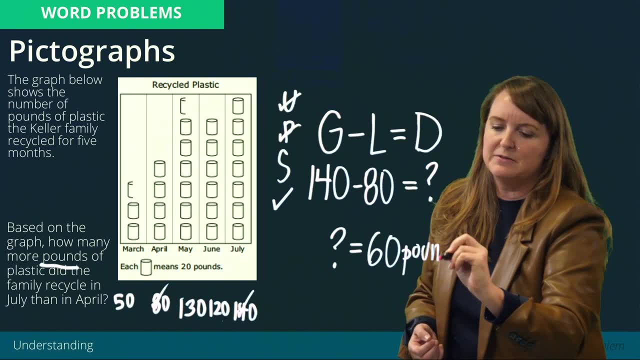 I'll go ahead and put in my signs. Let's think about how we should solve this. That question mark would equal 60. And what would be a good label for that? Well, I think pounds. That would be an excellent label for this word problem. 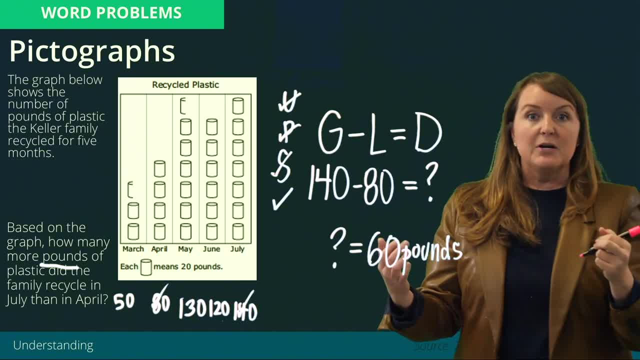 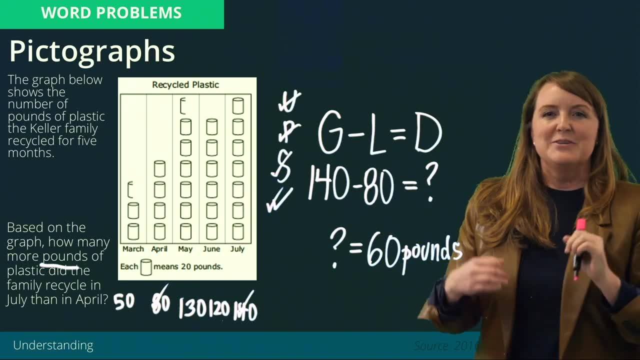 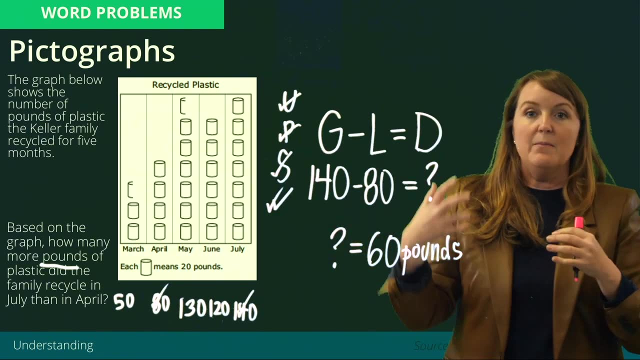 So what we did is we solved the problem, and then we want to go back and check our work. 60 plus 80 does equal 140.. Hurrah, We did it. So there, we used our word problem attack strategy, with a focus on the word problem schema, to help us set.